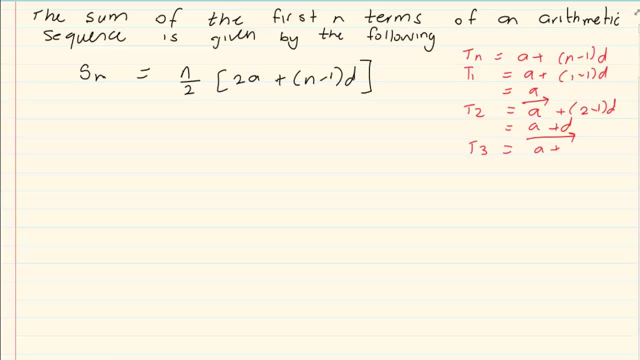 And if you go on, term 3 is equal to a plus 2d. Now we can go on, So I can go on with this and eventually I can come to the last term. Now the last term would be: if you notice, You will notice that a, when it was 1, then the d was 0.. When it 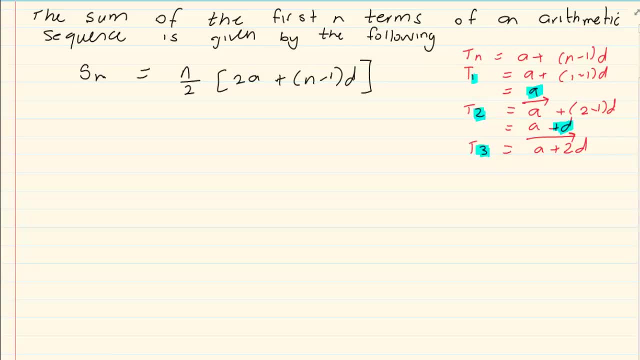 was 2, the d was 1.. When it was 3, the d was 2.. So what I am doing is I am decreasing by 1 every time. So if I have tn, it would be a plus n minus 1 d. 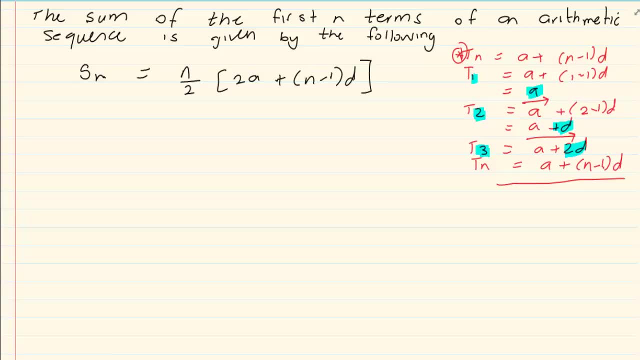 Alright, now why is this relevant? If I were to do sn Now, you would have to prove this theorem. Ultimately, this is what you want to show: That this is true. This really is the formula. Now, how do we go about it? If I was doing sn, If I was doing the formula, 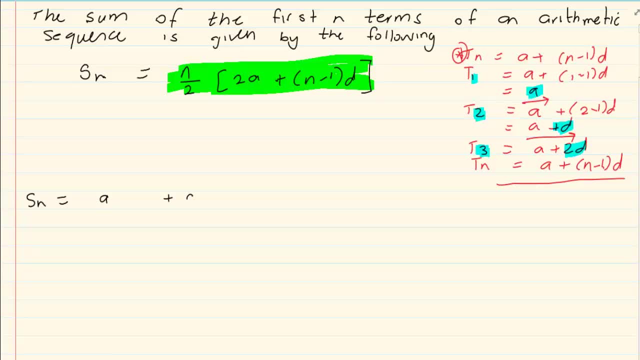 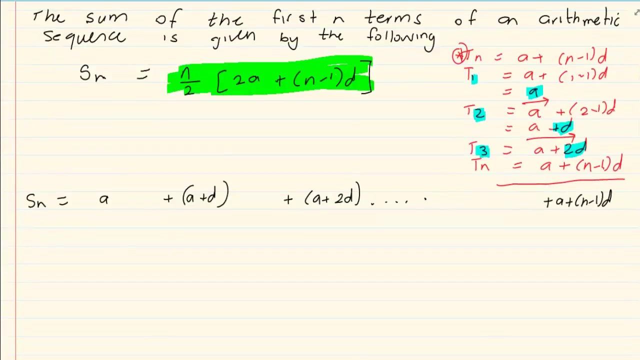 it would be a plus a plus d. So in other words, the first term plus the second term, plus the third term, And then I would go on and it would be the last term would be a plus n minus 1 d. If you wanted to write, if you wanted to write the second last term, it would be a plus n. 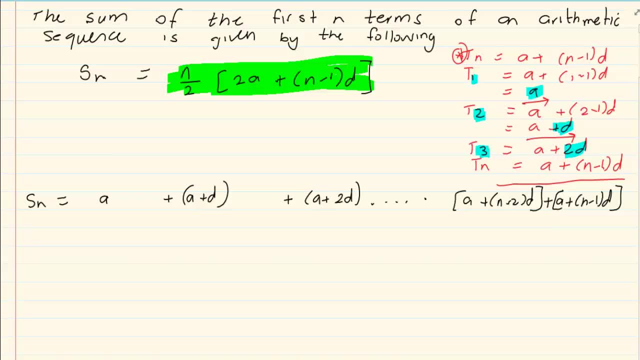 minus 1 minus 2 into d. Now this usually confuses learners, but think about it, right, If this was a 100, then this would be 99,, isn't it? Now, when we said we said 3 and then it's 2d, it dropped by 1.. Am I right? So the last term would be: whatever the term? 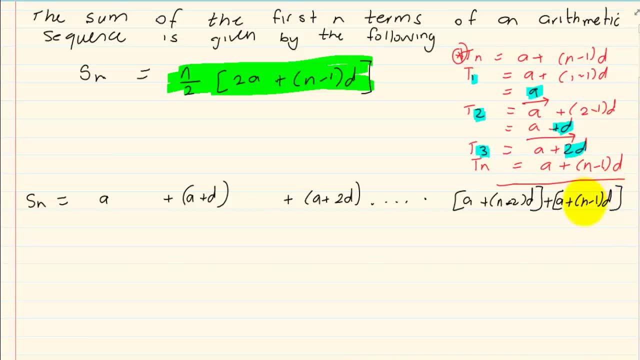 is, If it's term 100, then it would be 99d. So 100 minus 1 gave me 99.. Alright, But if it was the second last term, then it would be 98d, So it would be 100 minus 2.. 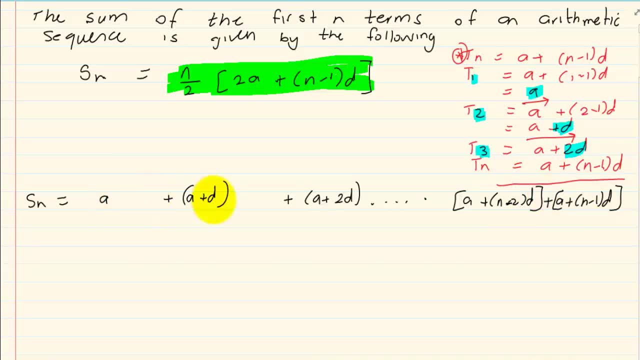 So it's decreasing, Just as here it's increasing. the d's d is plus 1, plus 1, plus 1.. So I'd have no d, I'd have 1d, I'd have 2d, and it goes on. It decreases. It would be minus 1,. 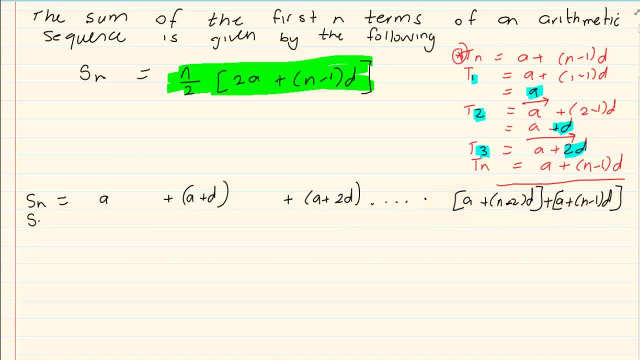 minus 2 and continue. Now, let's say, I did sn again, But I'm doing it backwards now. So I'm starting with my a on this side And then I'm gonna have a plus d, Then I'm going to start. what's the last term here? 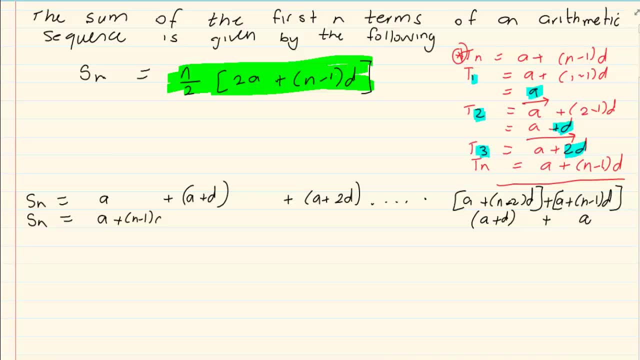 So here I'm going to have a plus n minus 1, d, And the second one will be a plus n minus 2d, And we can go on. Right Now, let us go through this. You understand how I got a. 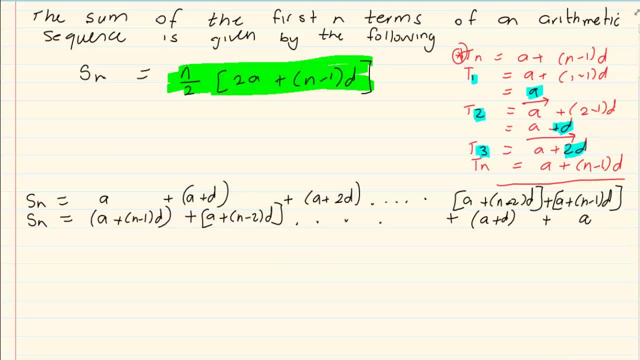 a plus d, a plus 2d, And we continue till forever, till the last one is a plus n minus 1d. Now I'm reversing it, I'm going backwards. So my last term is a. My second last term is a plus d. Can you see? I'm writing the same things down. Then I've got a. 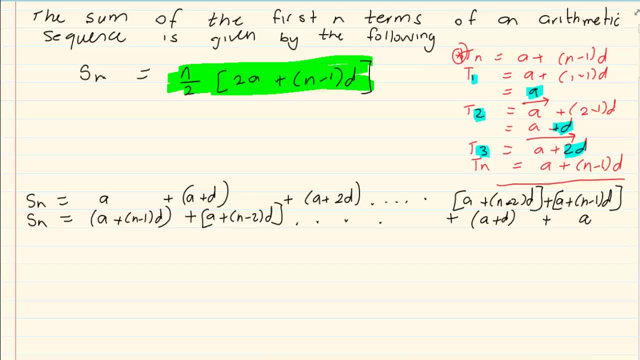 plus n minus 2d, a plus n minus 1d. Now what happens when I add these two? So I'm going to add these two lines. So if I say what's sn plus sn, I'm going to end up with 2sn. 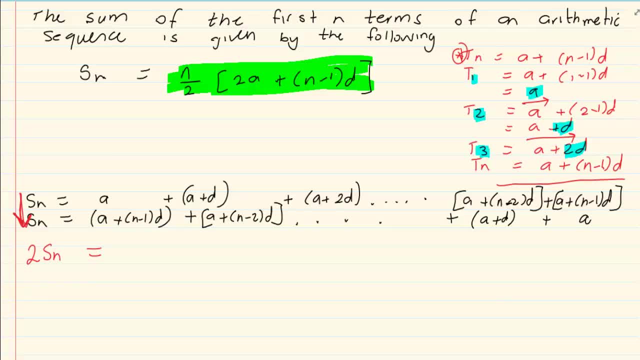 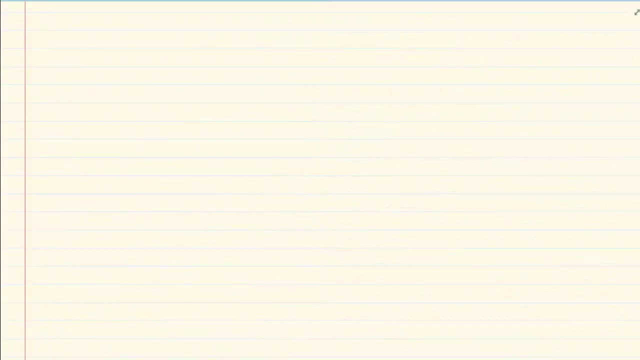 But what happens to these terms? What happens when I start adding a plus a plus n minus 1?? Now, if we were to do it in line, you would see it easier. So what I'm going to do is I'm going to just write it down here for you, Right? So if I said what's a 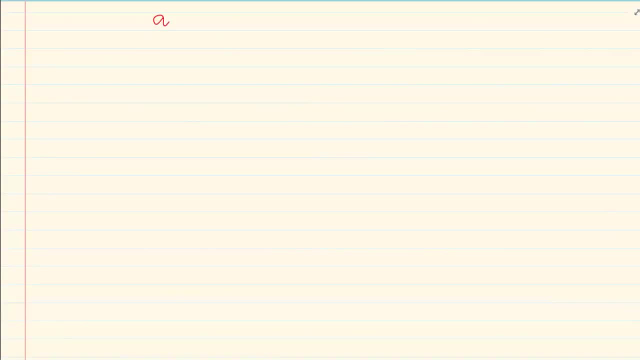 plus n minus 1d, I'm going to add these two lines. So if I say what's a plus n minus 1d, I'm going to say a. So if you look at it, we're doing it underline So you can see it easier. I have a. 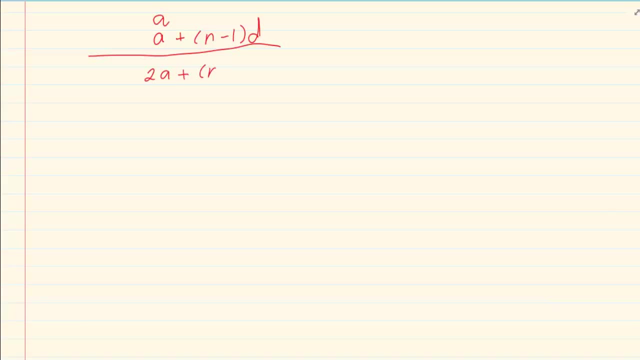 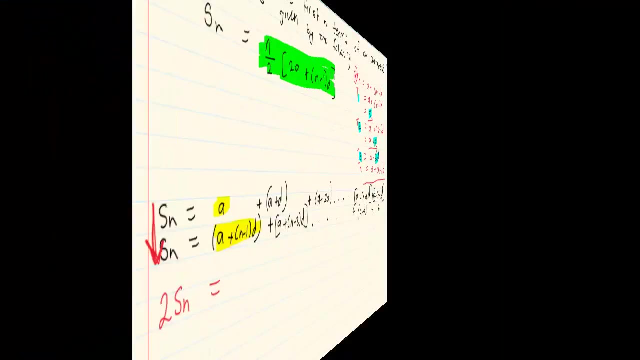 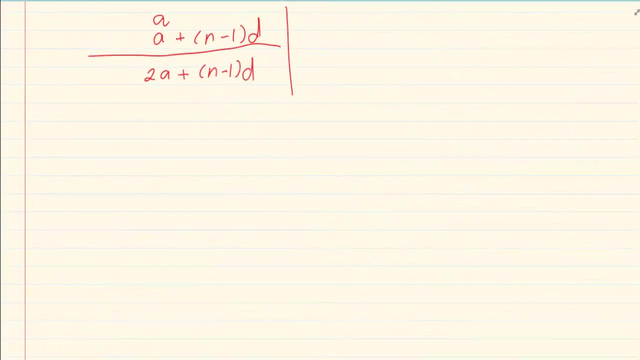 plus a is 2a plus n minus 1d. Right, Let's try another one. Let's try the second one, which is a plus d, and then a plus n minus 2d. So we've got a plus d plus n minus 2.. Right, So look at what you'd get. Now, this is a clever one. 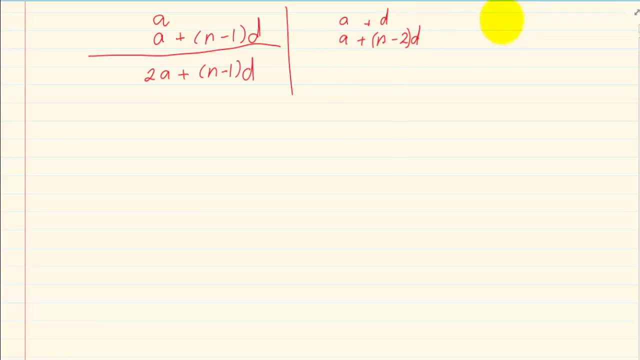 If you go, this would give me a plus d, But this would give me a Plus n d. Yes, Minus 2d, Because if you do distributive law, you end up with a. you'd end up with n d. 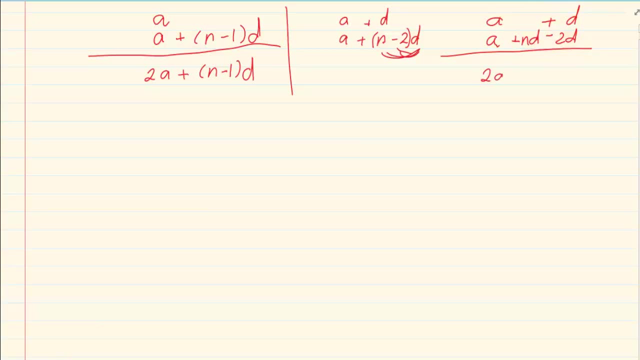 you'd end up with minus 2d. So this gives me 2a plus n d minus d. Now if we take out a common, we end up with 2a plus n minus 1d. So I took out d as a common. So if you take out d as a common, you're left with n minus. 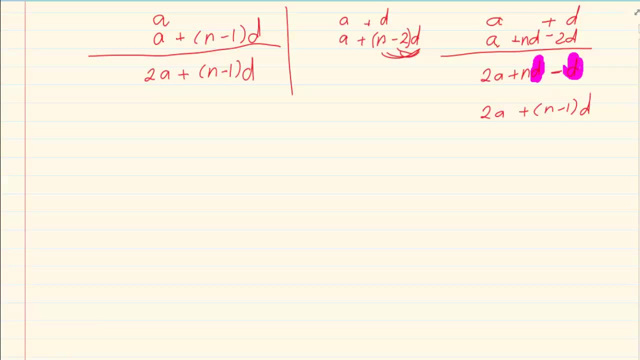 1. But what I want to bring your attention to is that look at these answers. They are the same, So you shouldn't frustrate yourself with how did they get 2a plus n minus 1d. How did I do this? If you know how to do the first one, then the rest is irrelevant. You're 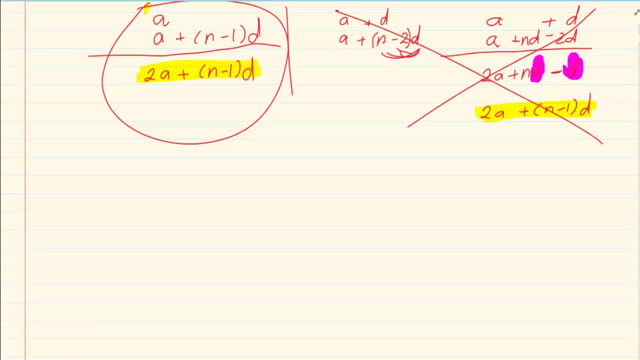 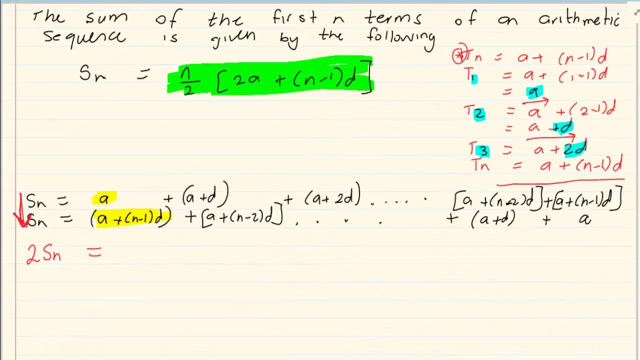 right, You don't need to know the rest. As long as you know the first one, you don't need to know the rest. So when you're doing this, you make sure that you know the first one. The one that I've highlighted is what's important. What would this become? It would 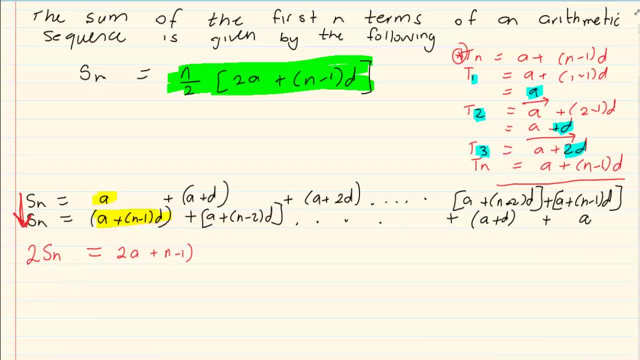 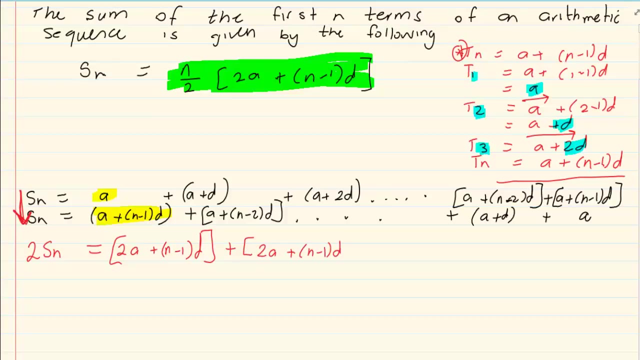